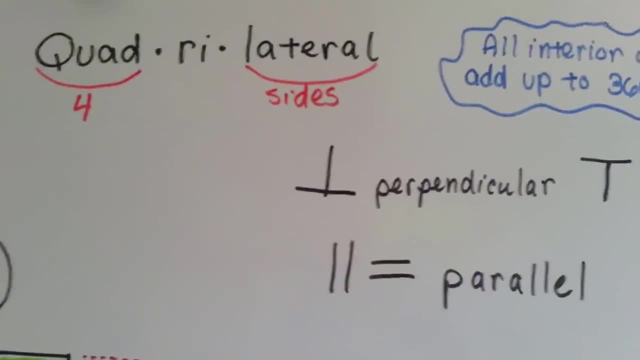 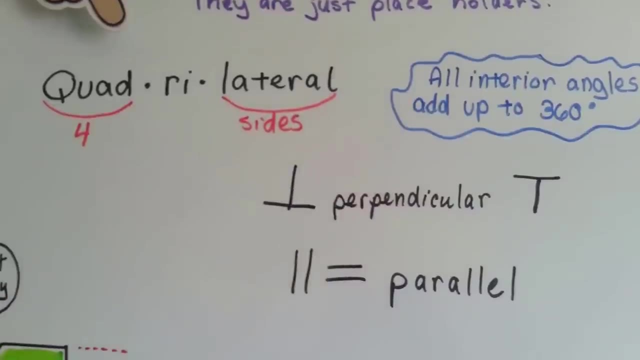 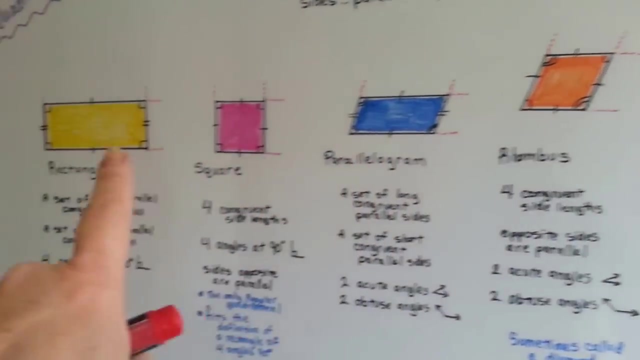 but they never touch. okay, The word quadrilateral actually means four sides, Quad means four and lateral means sides, And all of their interior angles add up to 360 degrees. Here's the five types, okay, And we're going to start with the rectangle. 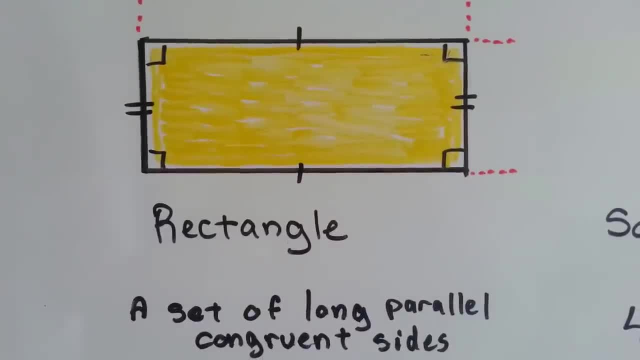 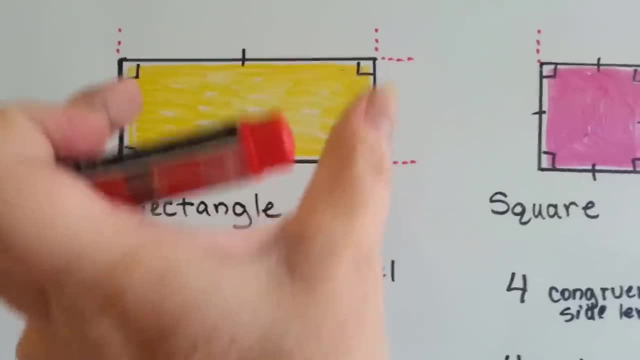 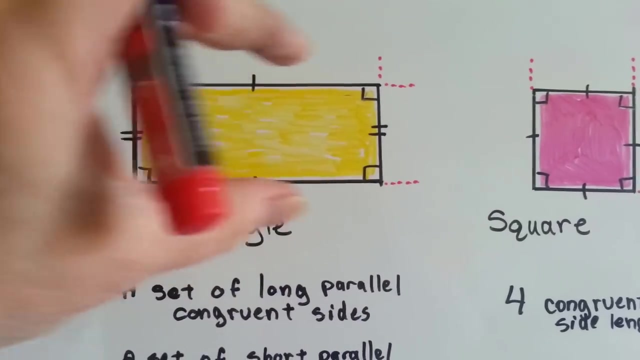 They have a set of long, parallel, congruent sides- see on the top and the bottom- And then they've got a set of short ones on the sides. This set has two lines because this is the second set that's parallel and congruent, And this has one little mark here because this is the first set. 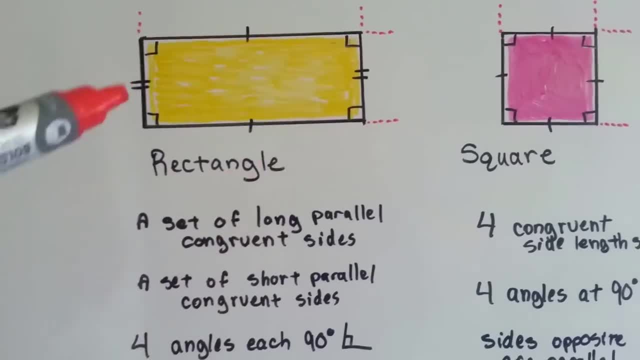 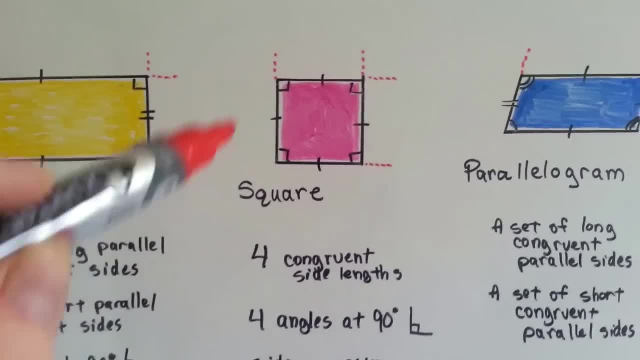 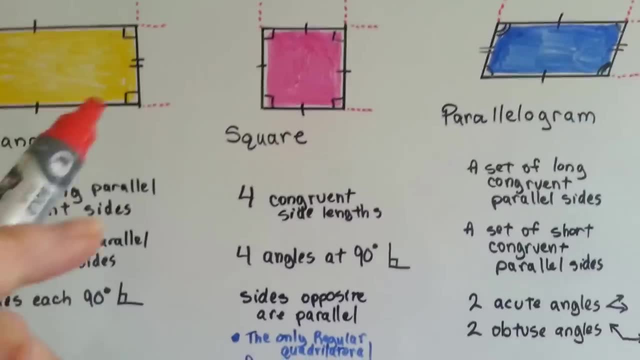 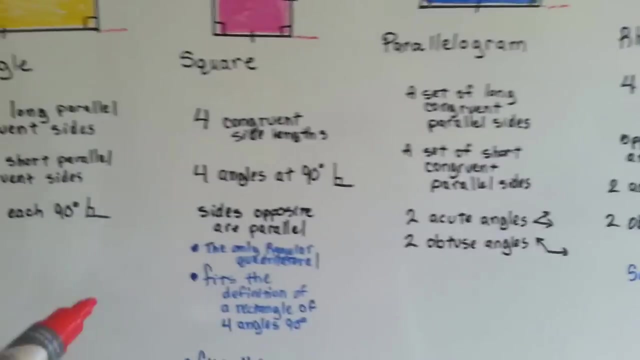 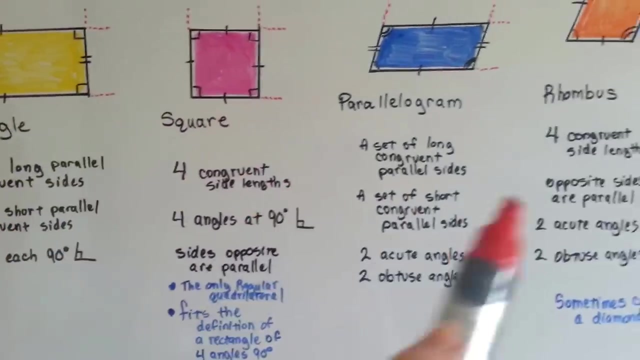 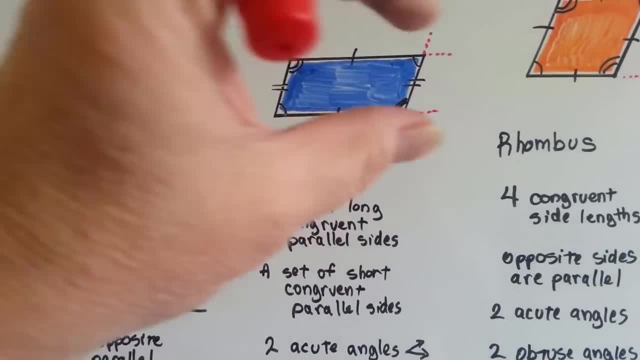 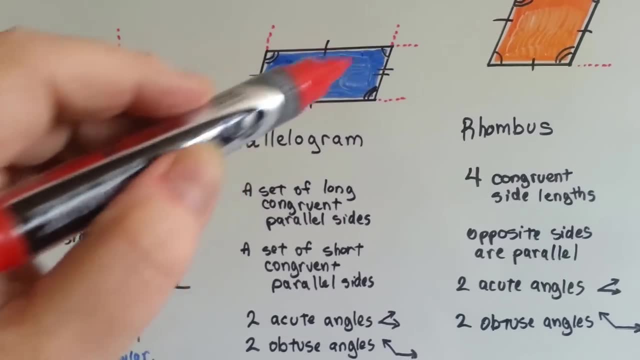 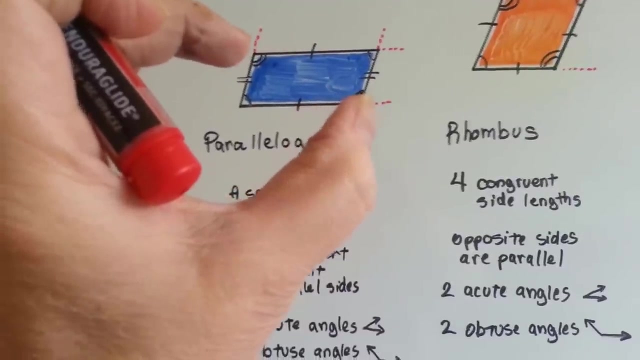 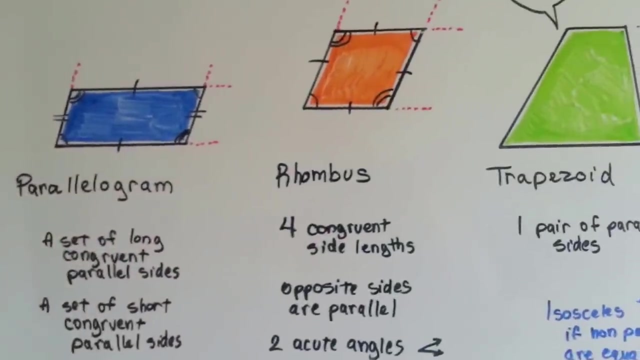 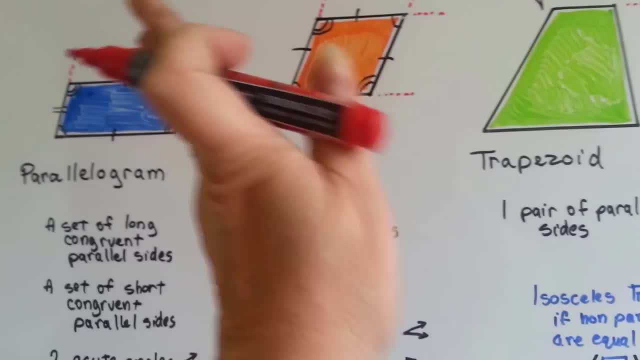 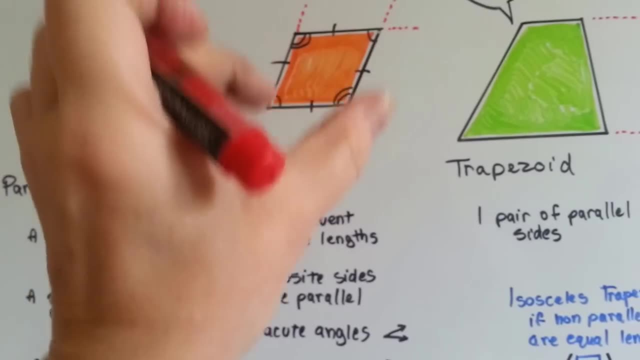 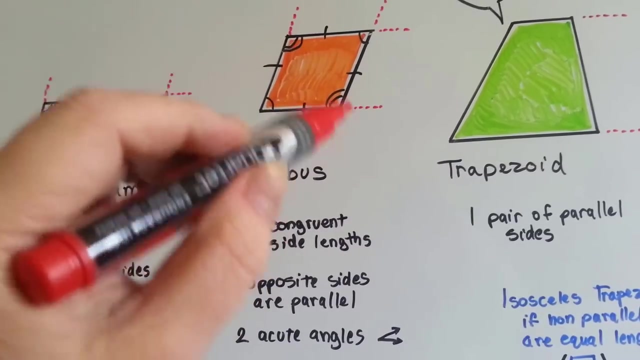 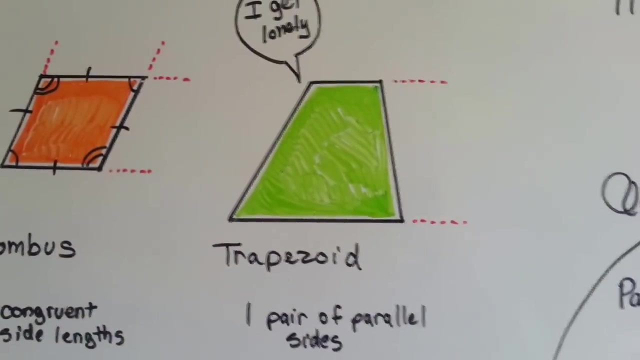 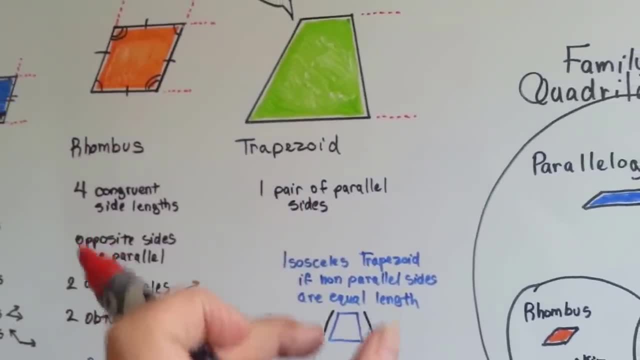 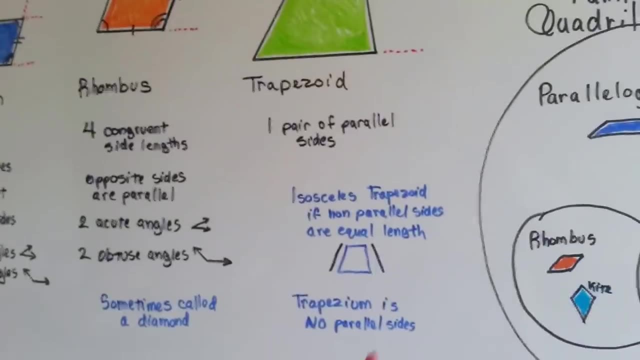 If it has equal side lengths on its non-parallel sides, if these are of equal length, then it's called an isosceles trapezoid. If it has no parallel sides, if these aren't even parallel, like they're kind of crooked, then it's called a trapezium. 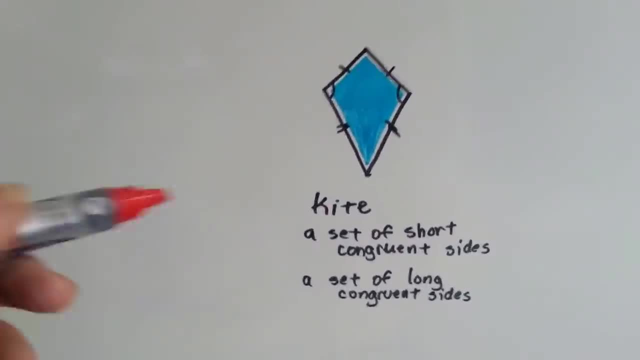 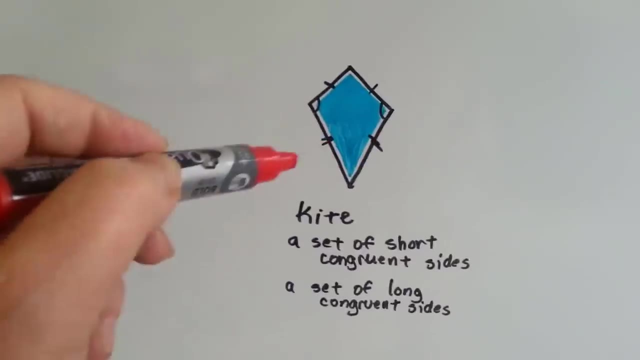 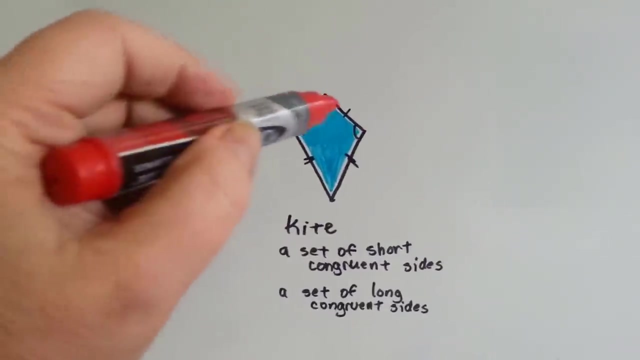 Now this is not supposed to be included in 5th grade math, but come on, It is a quadrilateral. This is the kite. These two top ones are congruent and these two bottom ones are congruent. It is a quadrilateral and you can see with the little marks how these are congruent. and then this is the second set that's congruent. 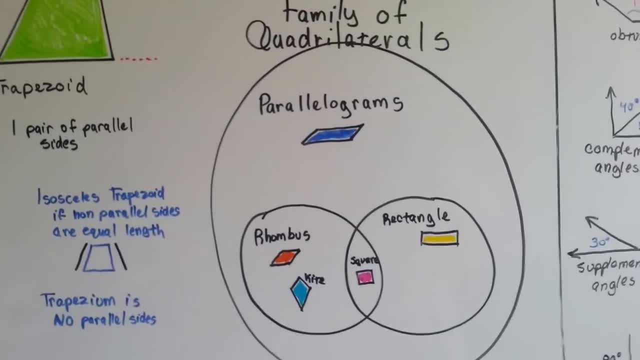 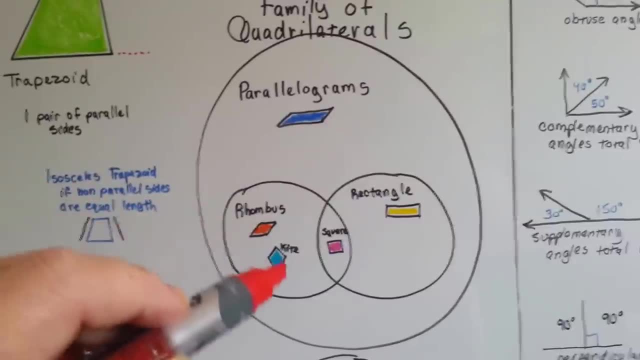 So in the family of quadrilaterals we've got a big family of parallelograms, and the rhombus and kite are in it together. The rectangle is over here and the square shares the traits of the rhombus and the rectangle. 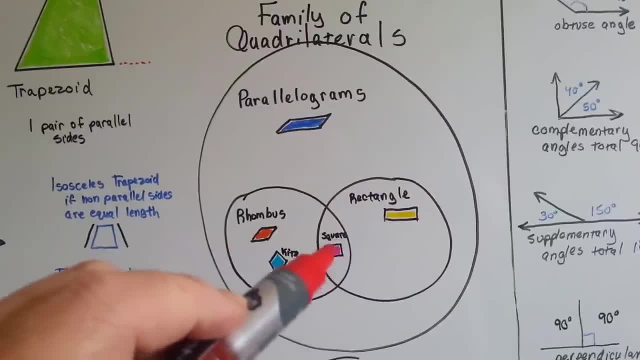 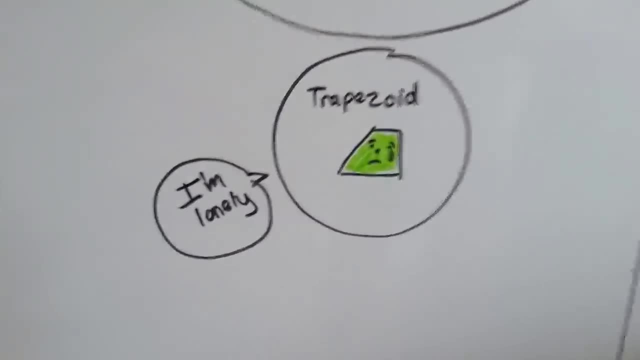 It's got the same side, It's got the same length like a rhombus, but it's got the 90-degree corners like a rectangle, so it's kind of both, isn't it? And then down here, look, we have our sad, little, lonely trapezoid who's crying because he's all by himself in his own little circle. 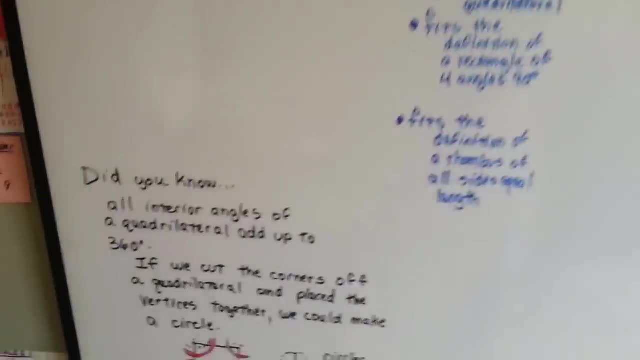 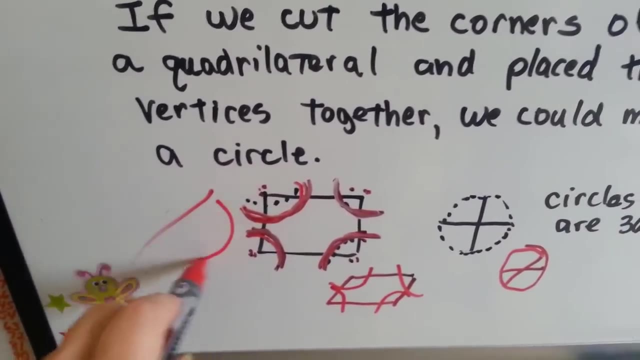 So I have a little art project for you to do, If you want to try this. get a sheet of school paper and on an arc, not straight, you've got to do it on a curve. okay, Cut the corners off of the sheet of paper on a curve. 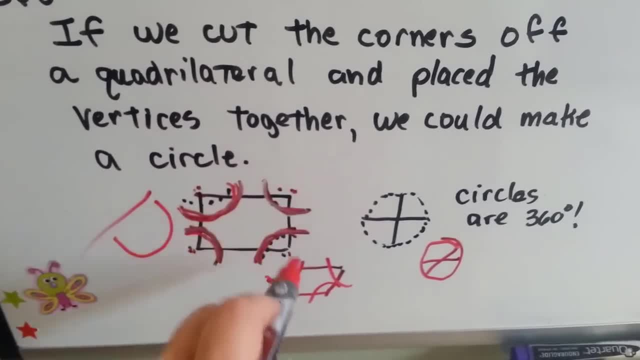 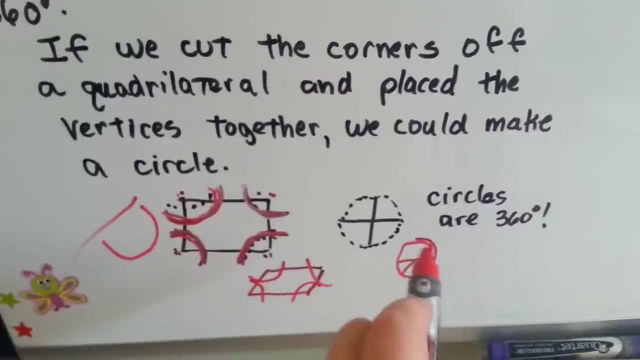 And then take each corner here, each vertice, and put it back to back like this, And it'll even work with a parallelogram, except your inside X is going to be on a slant like this instead of straight up and down. 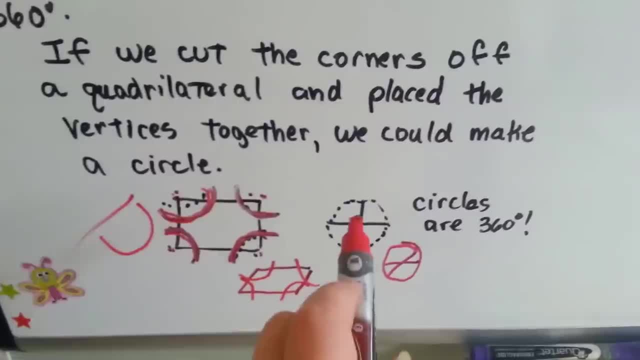 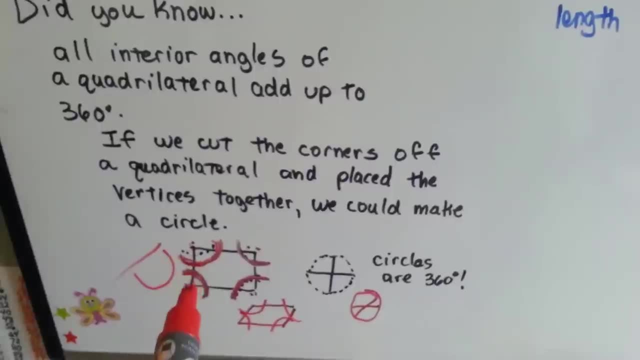 If you do it with a sheet of paper from school paper, you'll have the inside vertices touching like this and you're going to make a circle. It's because the interior angles of the quadrilateral add up to 360 degrees. if you cut these corners off in an arc, 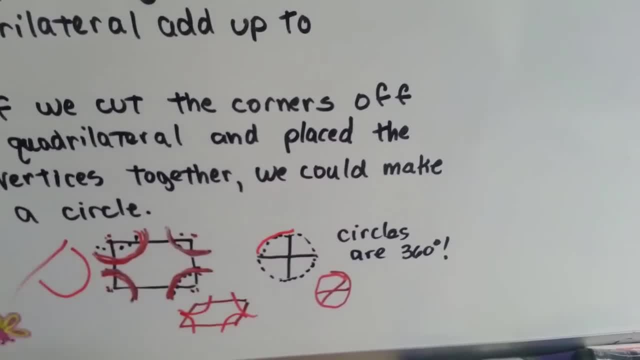 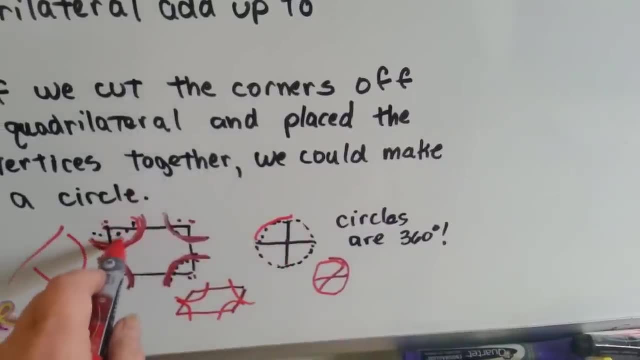 This arc is going to be an outside edge of the circle, see. And then this will be the corners that you put together, all the vertices in the center touching each other, see. So you're going to take this, flip it around and put it like this, see. 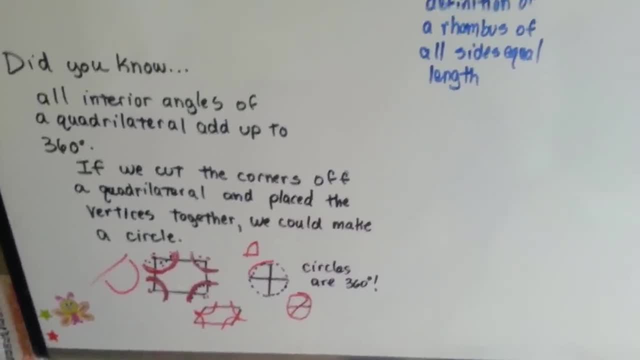 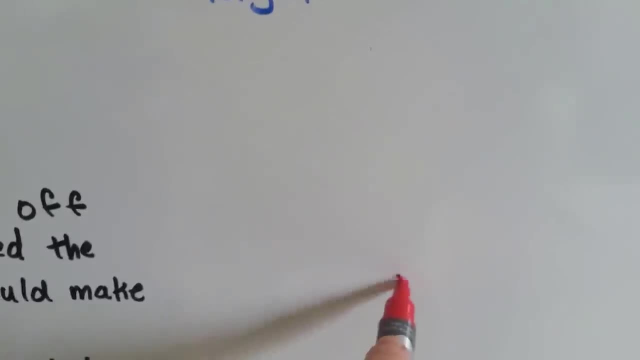 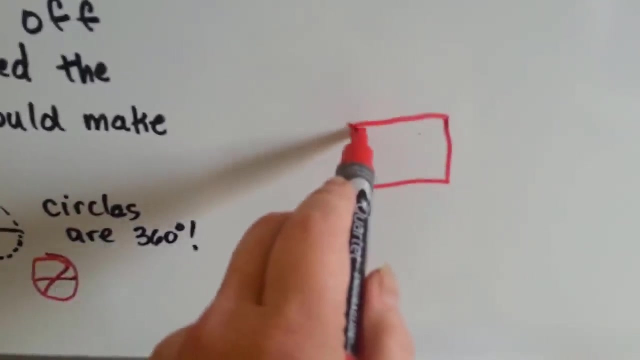 You'll make a circle, because circles are 360 degrees. Isn't that something? So, knowing you know what? Also, knowing that a quadrilateral has 360 degrees inside. we just talked about triangles. if you cut a quadrilateral in in an angle like that, you'll. 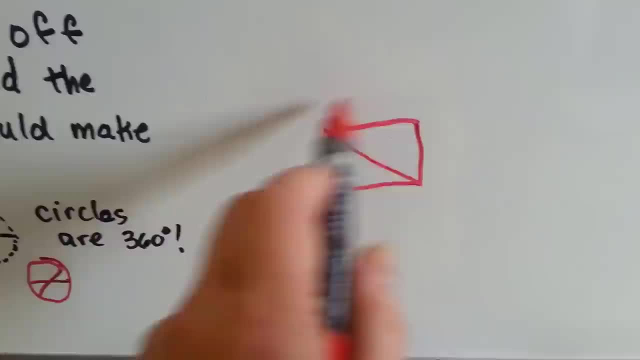 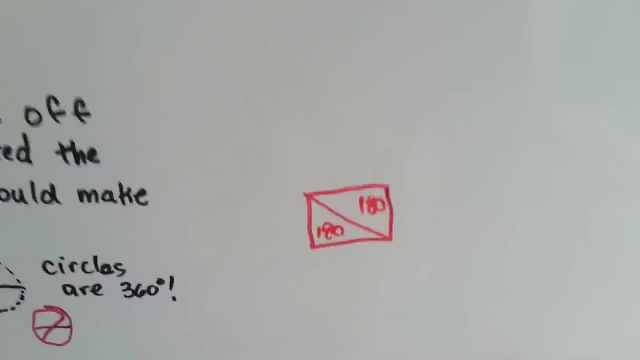 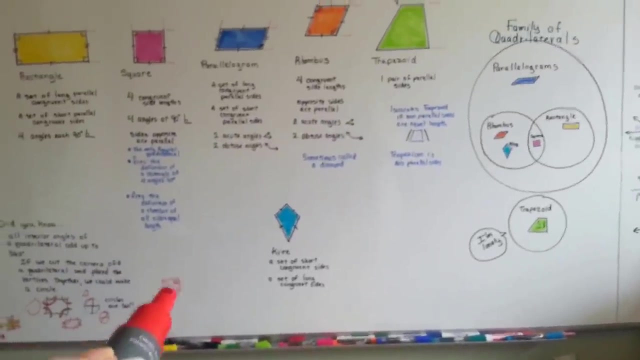 make two triangles, the whole thing inside is 360 degrees and we learned in the last video that this is 180 and this is 180, see, because triangles are 180 degrees inside. remember that from the last video. so two of them would make a quadrilateral and it would be 360, and it even makes sense. 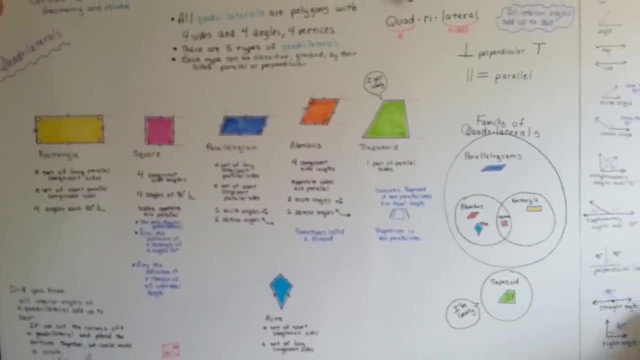 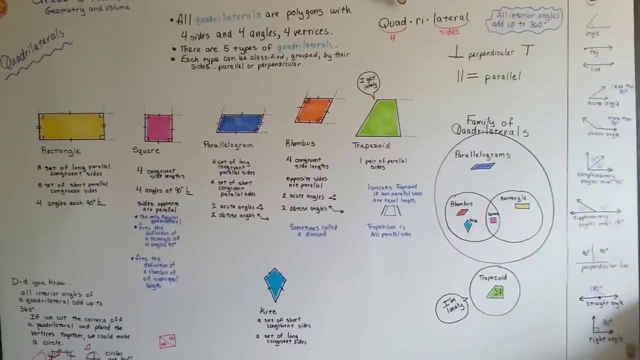 doesn't it, because 180 plus 180 makes 360. all right, we're going to continue talking about geometry and i hope this was educational and helpful and i'll see you next video. bye.